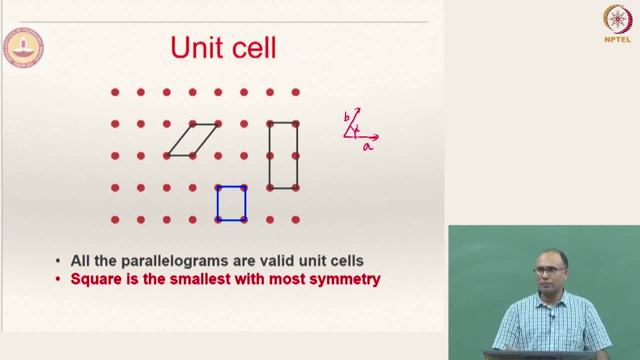 side is b and they are at an angle. a and b have an included angle of alpha. So now you can define as many number of unit cells as you want. So you can have conditions like a equal to b and alpha equal to 90 degrees. Then you will have a square unit cell. If 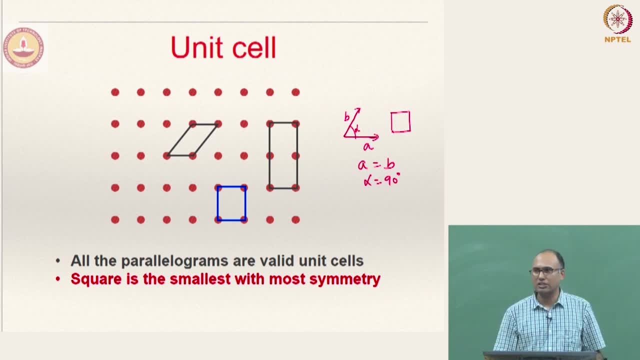 a is not equal to b and alpha equal to 90, then you will have a rectangular unit cell and so on. So when you have this small geometry and if you take this geometry and translate the geometry in the lattice direction, so lattice vector, So what will be the diameter? So, 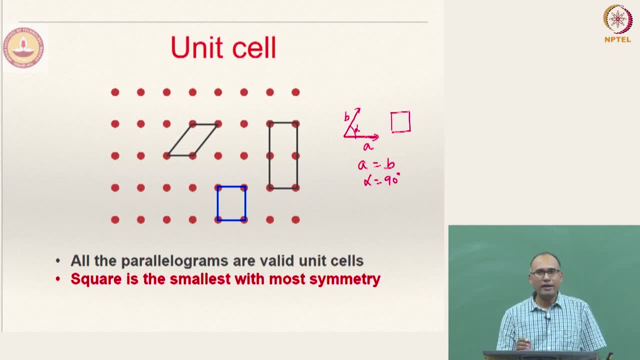 This is what is called lattice vector. and you take this geometry and translate it both in x direction as well as in y direction for 2D, Then it should fill the entire space. It should not leave behind any voids. Only then such a geometry qualifies as unit set. 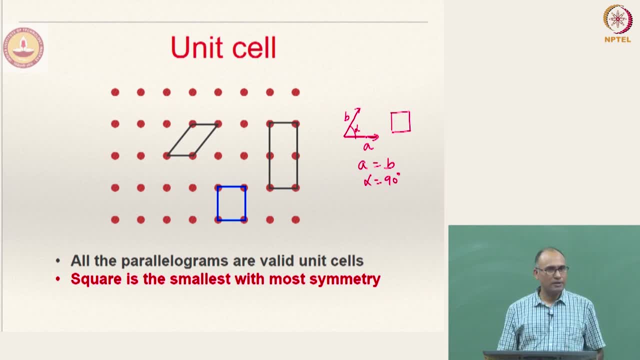 So now imagine having a triangle. can you fill the entire space of this particular lattice using a triangular unit cell of your choice without leaving behind any voids? Is it possible or not? Just by translation it is not possible. You will have to rotate the unit cell. 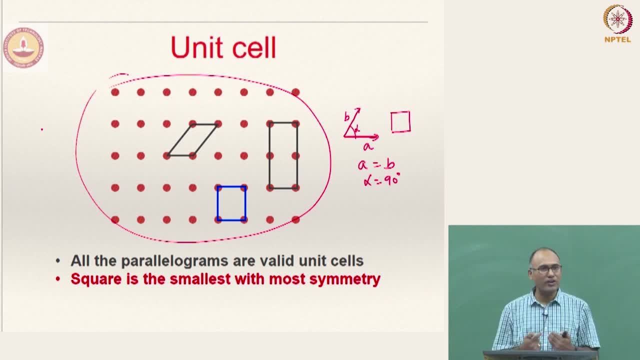 And hence your triangle cannot be a qualified unit cell, But it is for filling the space right. So in general, in 2D a parallelogram will be a qualified unit cell and in 3D a parallel pipe will be a qualified unit cell right. 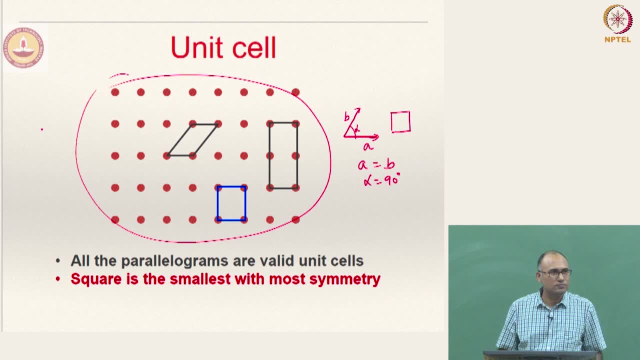 And what will be a unit cell in 1D? It will be a line. Line will be the unit cell in 1D. And then we have discussed the concept of primitive unit cell and non-primitive unit cell. right, What is the concept of, what is the meaning of primitive unit cell? 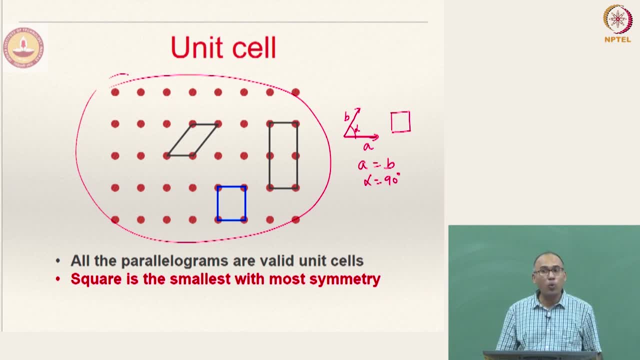 Primitive unit cell is the one which has effectively one lattice point associated with the unit cell. And if it is a crystal, then effectively it will have one atom or one molecule or one ion, depending upon what is the point that is sitting. We will talk about it in a moment, okay. 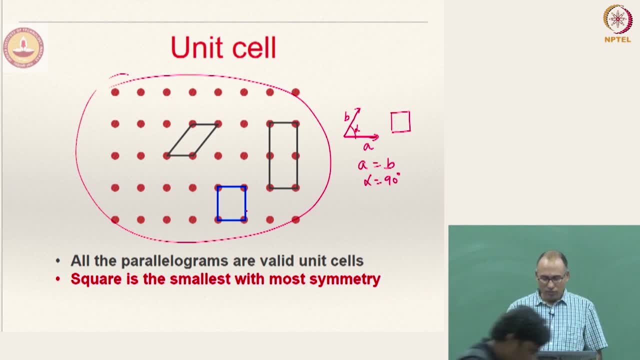 So here we have. this is the smallest unit cell, right with highest symmetry. So usually you choose the guideline is you choose the smallest possible unit cell as your unit cell of the lattice that you are looking at. But it is not a requirement. 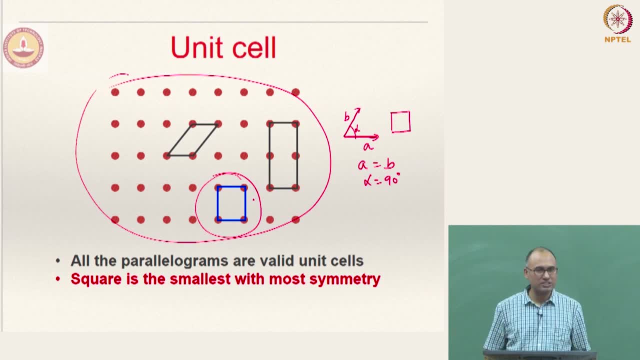 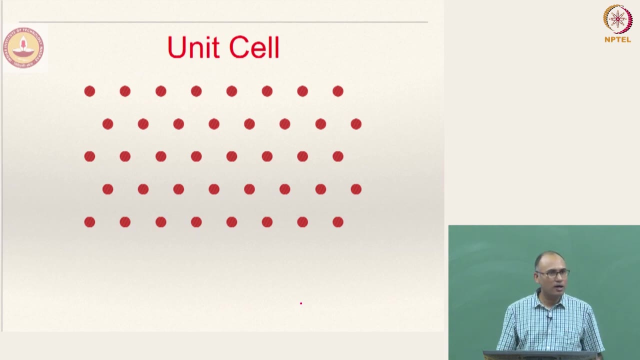 You can- actually, in principle, you can- choose infinite number of units. You can choose infinite number of unit cells, as we have shown, And then fill the space. okay, alright. So again, previously we have seen a rectangular unit cell and hence you have a different set. 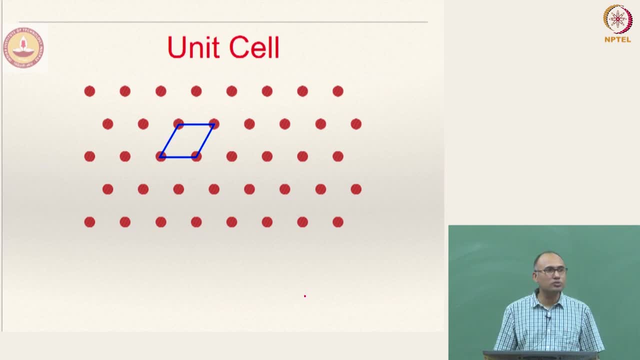 of unit cells that you would get Here. it is not possible to get square as a unit cell Because the way the lattice points are arranged it is not possible to get square as a unit cell. So you have to choose something else as your appropriate unit cell. okay, 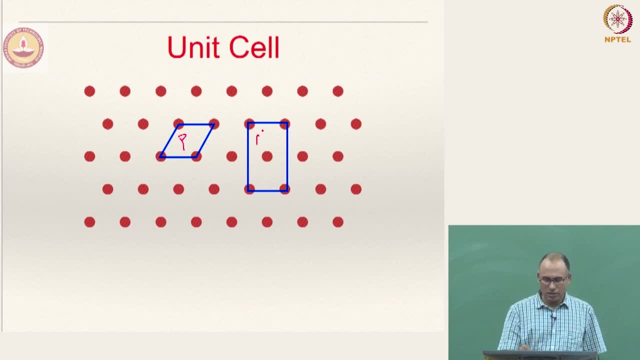 And here you have seen, this is a primitive unit cell. this is a non-primitive unit cell, right? Why is it a non-primitive unit cell? Because, effectively, it has two lattice points per unit cell and hence it is a non-primitive. 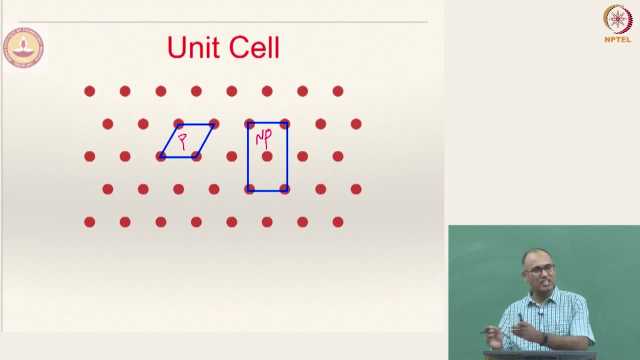 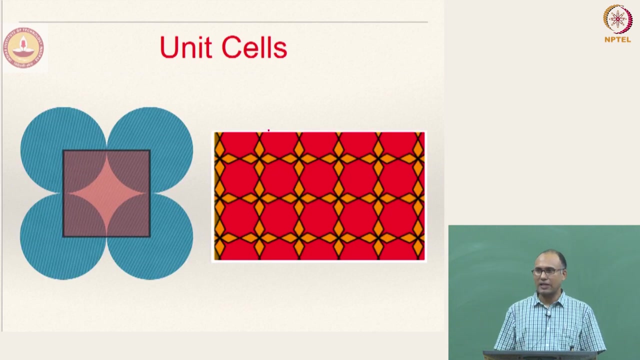 unit cell, So you can also choose non-primitive unit cells to fill the space. There is no problem with that. Alright, so this: I think we have looked at this concept. so you have this styling and then a two-dimensional map and you are trying to see different kinds of what are the different? 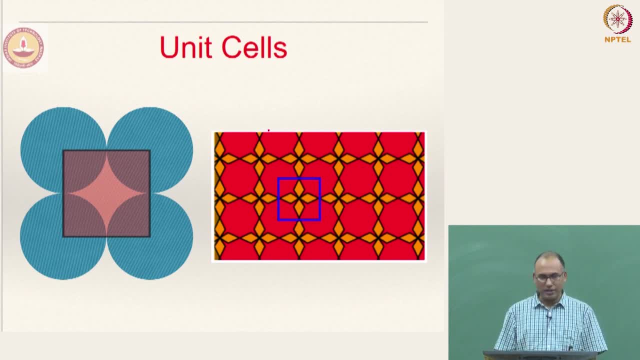 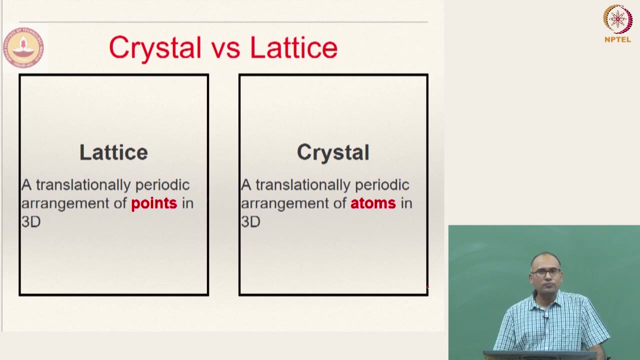 unit cells that are possible. So you can, we have already identified this as a one possible unit cell and then that geometry as another possible unit cell and that geometry as another possible unit cell. Okay, Thank you. Alright, So now we have only looked at the definition of lattice, right? 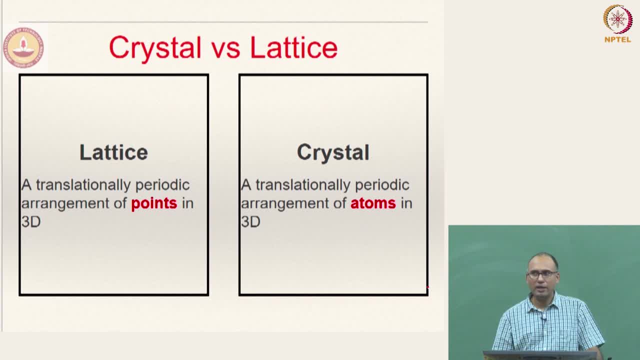 What do you mean by crystal? What is the difference between crystal and a lattice? So lattice, by definition, is a translationally periodic arrangement of points in three. That is what we have seen. right when we saw the Cambridge wall example, what we did. 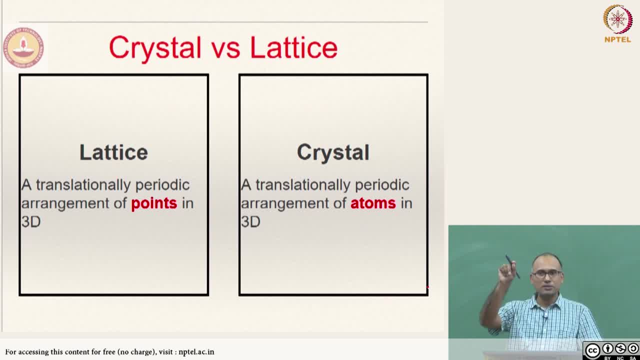 was. We have identified bricks, Okay, We have identified bricks that look identical right, And then it is a two-dimensional space and we have identified those points and then removed the brick brick wall, And then the set of points is what we call lattice. 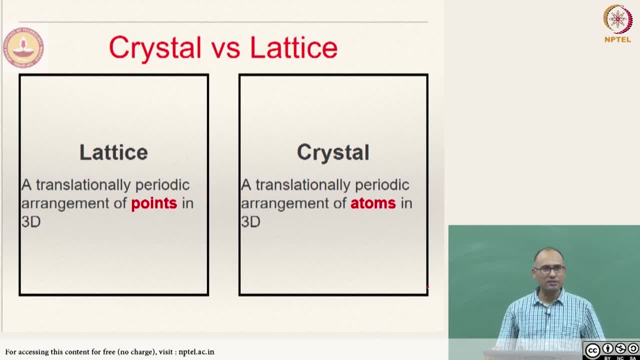 So it is basically a translationally periodic arrangement of points in 3D in general. But if you are defining a 2D lattice, that will be in 2D. If you are defining 1D, then it will be 1.. 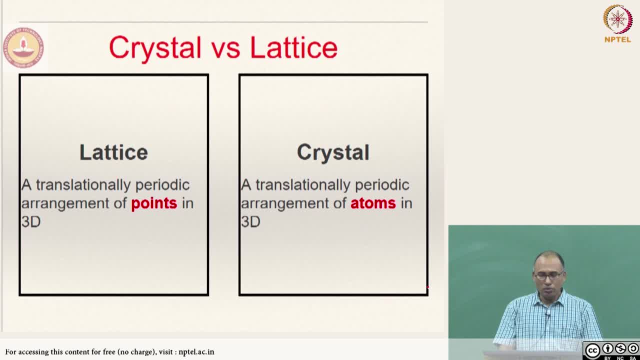 Clear Now what is crystal. So the only set lattice, when we are defining a 2D lattice, that will be in 2D. If you are defining 1D, then it will be 1.. Clear Now what is crystal. 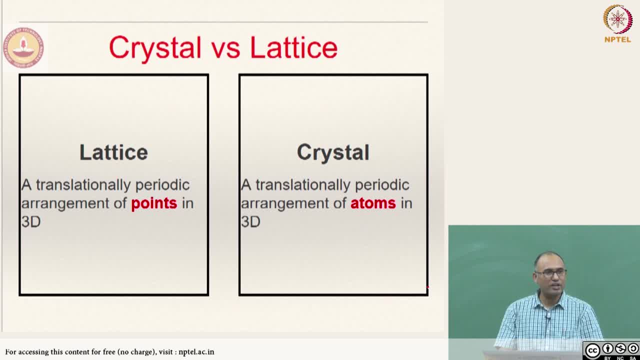 So when we are defining lattice we only set point right: periodic arrangement of points. These points can actually be occupied by some real stuff. If they are occupied by atoms, ions or molecules, then that becomes a crystal right. So a translationally periodic arrangement of atoms is what is called in 3D is what 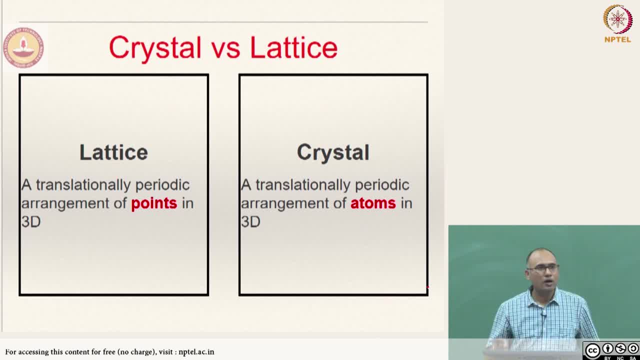 is called a crystal. Sometimes a crystal need not be Okay. It can be of a pure metal, but it can be of an alloy. So that means instead of having, if you look at iron crystals, so only iron will be there. 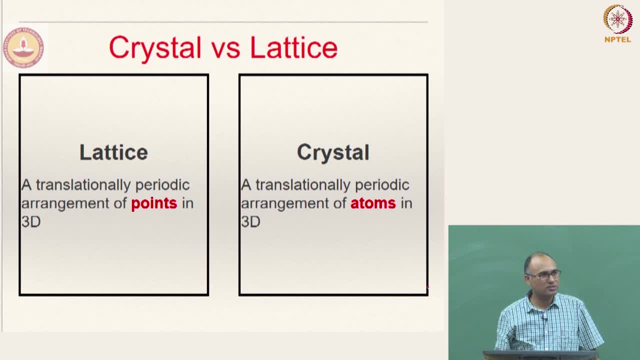 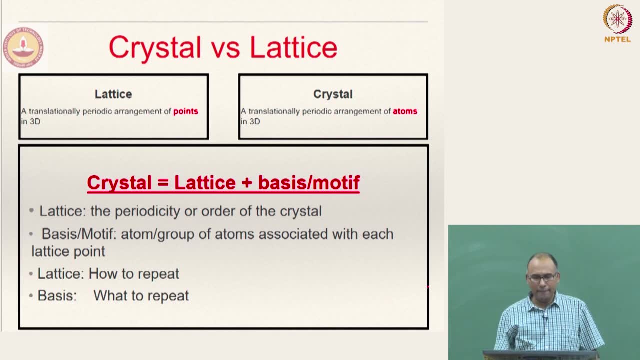 But if you want to look at iron oxide, Fe2O3 will be there at the lattice. That is the idea. Okay, So to reinforce this idea of the correspondence between lattice and crystal, a crystal is nothing but lattice plus a motif. 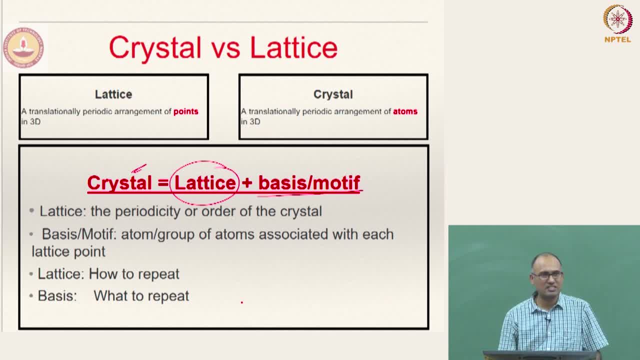 Okay, So that is the idea. Okay, So lattice is nothing but lattice plus a motif or basis. That means whatever sits on the lattice points is what is called motif. Then, the moment you add motif, then that becomes a crystal of that motif. 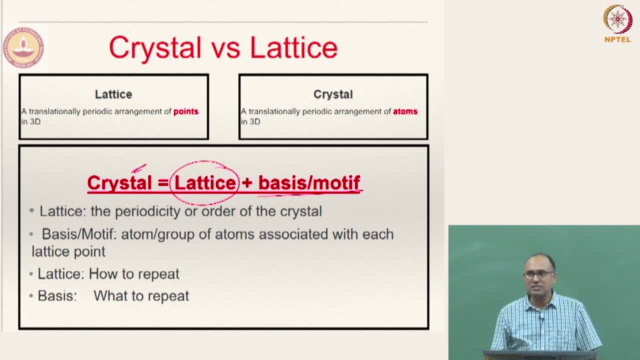 Right. So what lattice tells you is how to repeat the points, Right. So the moment you remove, you have, we have removed the brick wall. you have got the points. Now, once you have the points, you can actually construct the entire brick wall, because it 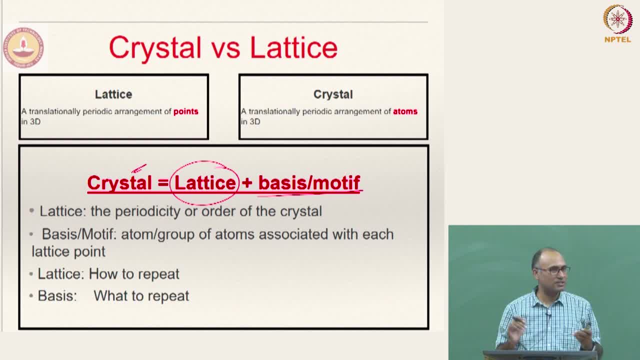 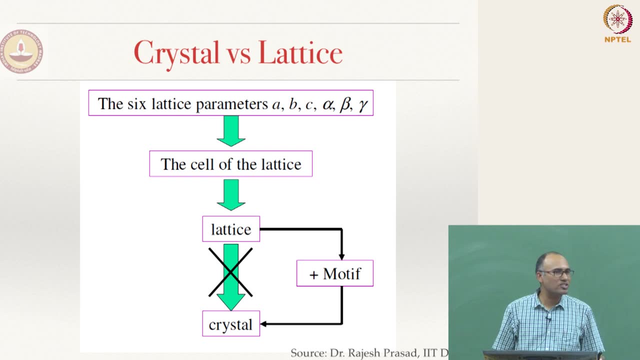 told. it told you, But it showed you how to repeat these points. So lattice tells us how to repeat, And what does basis or motive tells us is what to repeat. So in 2D we have seen how many lattice parameters are required in two-dimensional situation. 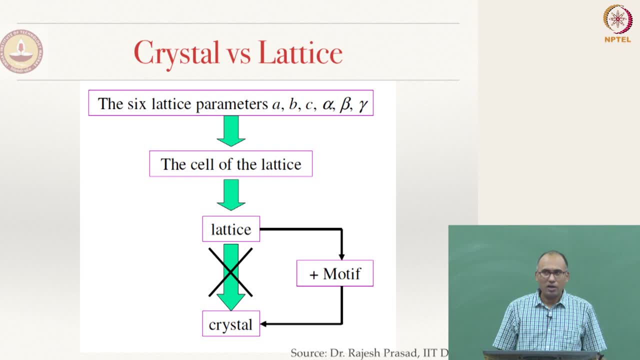 to define a lattice or to define a unit cell. I am sorry to define a unit cell 3, a, b and alpha. So in 3D you have 3 edges and 3 angles. so a, b, c, alpha, beta, gamma right. 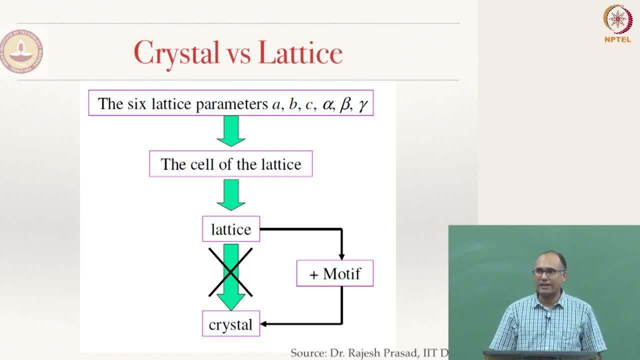 You have these 6 lattice parameters and then you get the cell of the lattice right. that is the unit cell. Please note that unit cell has nothing to do with the size being unique, okay, So unit cell size need not be 1.. 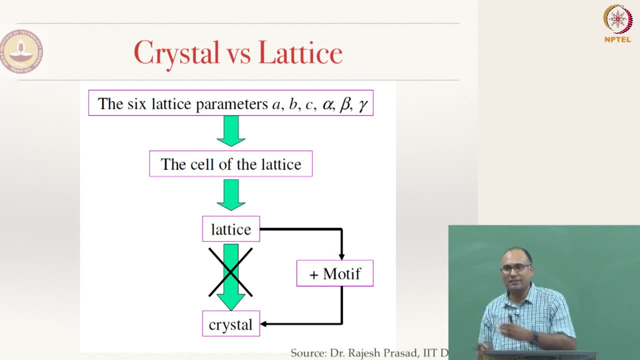 It is the basic unit that is being repeated, right, It is not about the number 1.. It is the basic unit that is repeated. that is why it is called unit cell. okay, And then that cell of the lattice. you have this cell of the lattice and then from there. 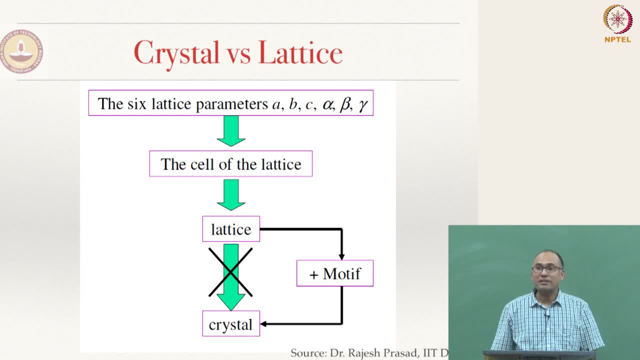 you can actually construct the lattice, But that is, that will not be called a crystal. The lattice cannot be called a crystal. You can only call lattice as crystal when you add a motive to that. okay, So how do we understand that? 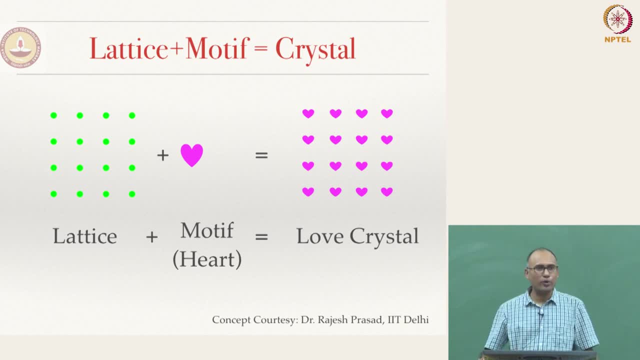 So let us say these are units, Okay. So you have your set of points- lattice point, okay. And then you have your heart as motive, okay, And you put heart at each and every position, and then you get something called love crystal. 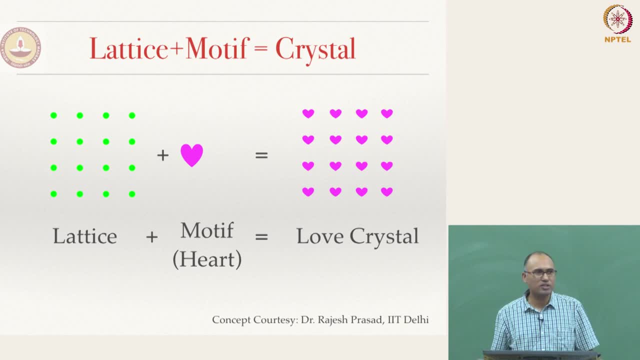 or heart. You replace that with football, then you will get football crystal. You replace that with theater, you will get theater. you can construct anything right. So that is the idea. so now you replace that and then you know what? clearly the difference. 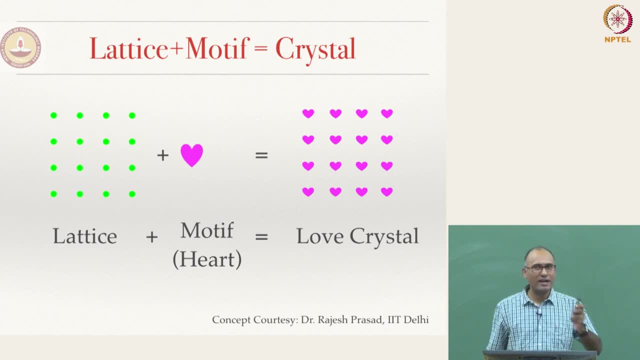 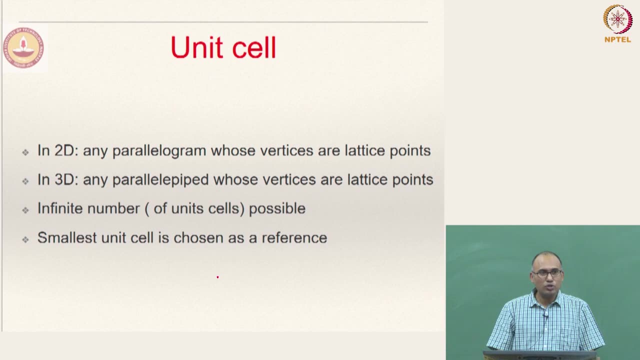 will be in how do you distinguish the definition of a lattice and a crystal right? all right. So in summary, in 2D, any parallelogram whose vertices are lattice points in a unit cell. in 2D you will have any parallelogram whose vertices are lattice points.